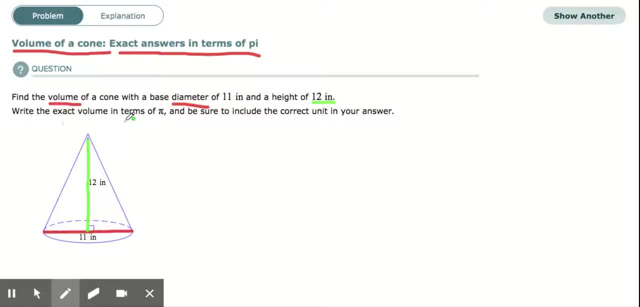 is 12 inches. Write the exact volume in terms of pi and be sure to include the correct units in your answer. So I think a lot of people struggle with this. um, with the finding the volume of pi. It's very common that people find the volume of pi in the form of a cone, because they don't really 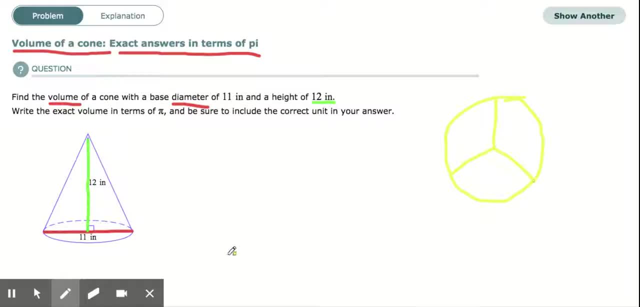 understand where the formula comes from. Well, let's take a circle and let's cut it into thirds, into three equal parts. When we do that, um, and then you just take one of those parts, Let's get rid of these two. So take away one third and then take away this other third. Do you see how we have? 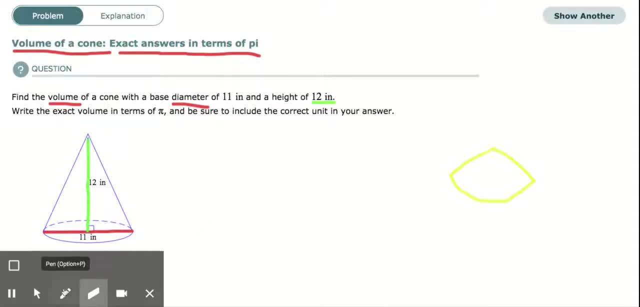 this shape. Now picture: if we took this and we rolled it up, it would make a cone. Do you see that? So this really represents a third of the entire circle and that's where the third in the volume formula comes from. So the volume, 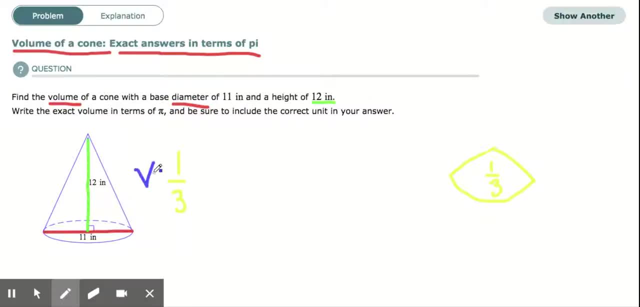 let's do this in a different color. the volume is equal to one third of the area of the base, and the area of the base is a circle, so it's pi r squared times the height. Okay, so just be careful: This base it's not just 11, it's actually the area of the base right here. 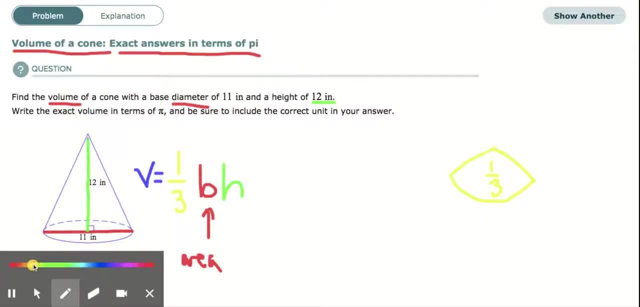 Okay, so let's go ahead and write this out. So volume equals one third of the area of the base and the area of the base is one third of the area of the base. So the base is a circle. so we want to go ahead and write the area of a circle and that is pi r. 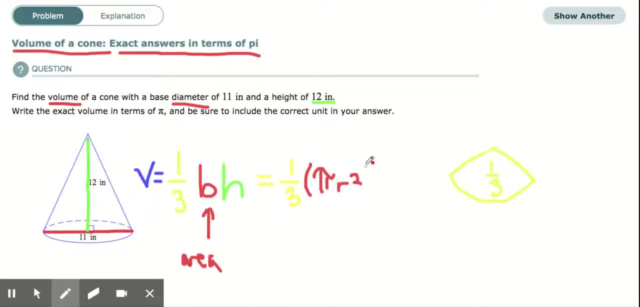 squared, That's the formula for the area of a circle, and then times the height, and the height was given to us, that's 12.. And the only thing that's tricky about this is that we don't have the r, we have the d, the diameter. 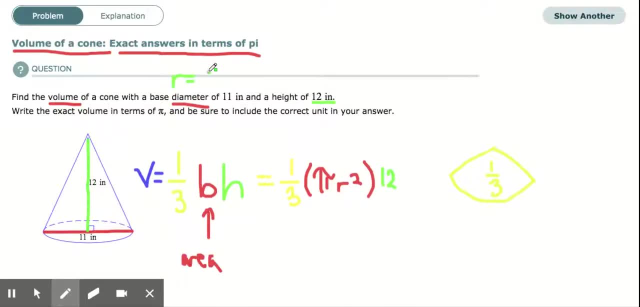 But the radius is equal to half of the diameter, or you can think of it as the diameter divided by 2.. So this radius is halfway across the circle. If the whole way is 11,, that means that the radius is five and a half. So what we're going to get here is 5.5 squared times pi. 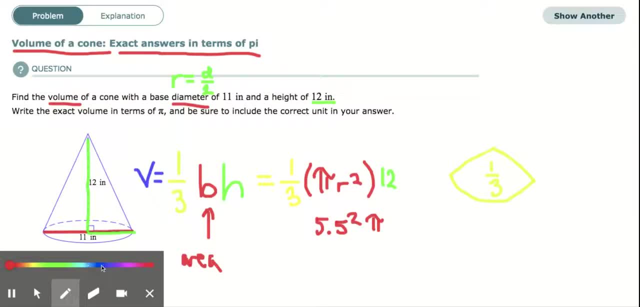 Times one third and times 12.. Well, if you do one third and you take a third of 12, that's the same as 12 divided by 3, right? So when you put those two things together, you're just left with 4, right. 12 divided by 3 is 4.. Now, what's 5.5 squared? 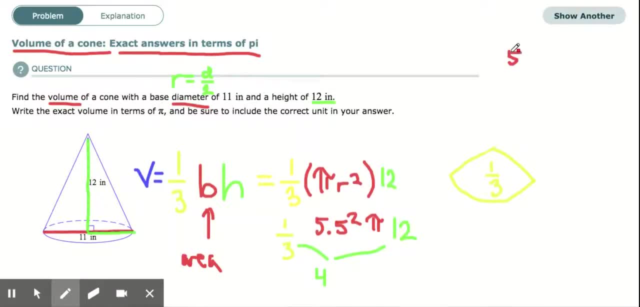 Let's go ahead and do this out: 5.5 squared, What would be times itself. So let's see: 5 times 5 is 25.. And then 25 plus 2 is 27,. right, And then we're doing the tens. so now we put a zero here And you would get the same thing again. 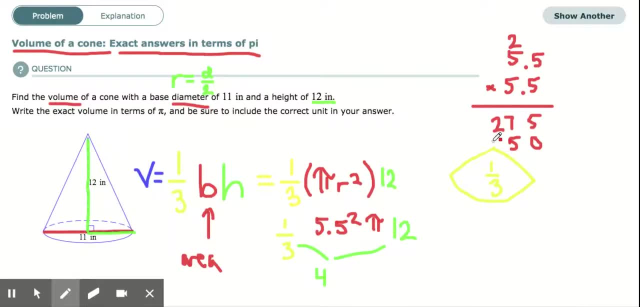 So you'd get 5, and then you'd get your 7, and you'd get your 2.. So when we add this up, we get 5,, 12,. so carry the 1.. That would make 10,. carry the 1.. 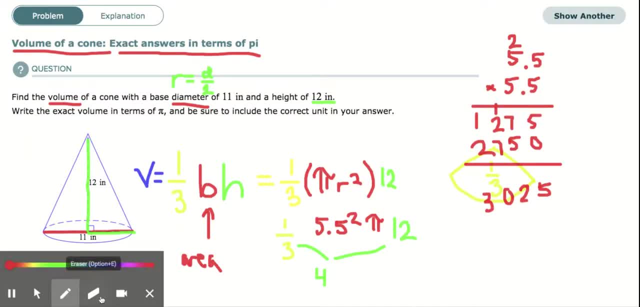 So this is 30, and then there's decimal points. right here It's one decimal point, two decimal points. so we go over two decimal points 5 times 5.5. squared is 30.25.. So this is really 4 times. 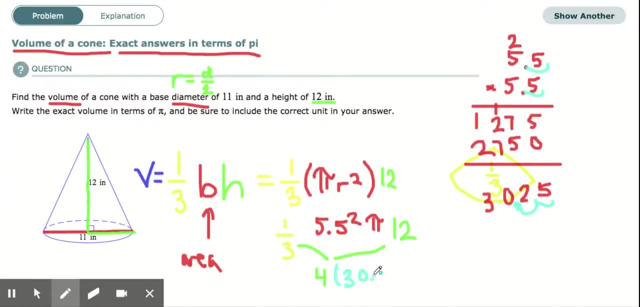 30.25 pi, All right. well, let's see What is 4 times 30?? Well, that's 120.. And what's 4 times a quarter? Well, that's just 1.. So this is actually equal to 121 pi. And then let's think: